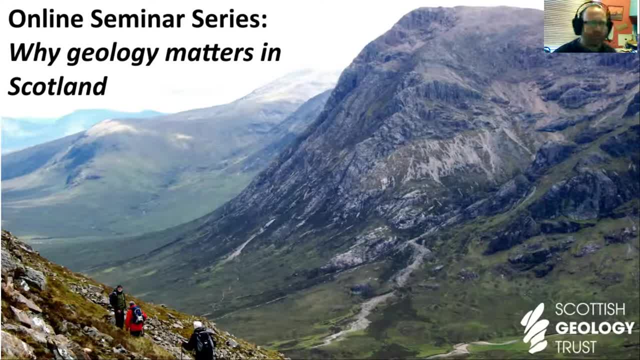 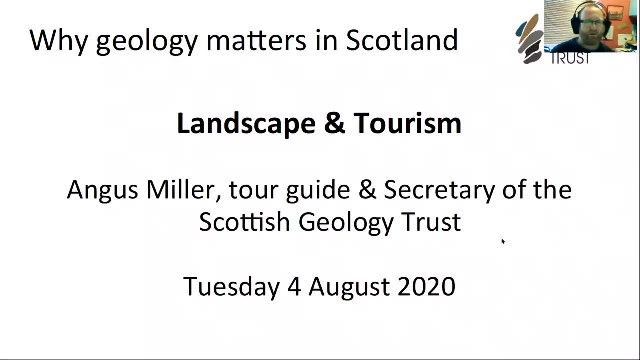 Let me get started, and thanks very much for for coming along today. What I wanted to just generally talk about is landscape and tourism in Scotland and in relation to Scotland's geology. and well, I said the seminar series would be all presentations by experts and of course, that. 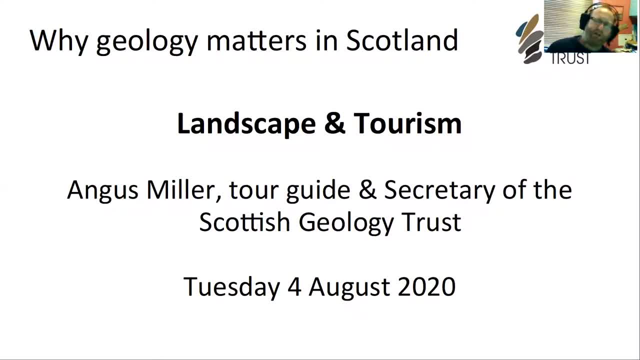 means I'm calling myself an expert and I'm not sure if I am, but I've been leading geological tours in Scotland for 20 years now with various groups. a lot of day trips and holidays for people from Britain who are interested in geology, but also, as I'll explain, a bit more kind of 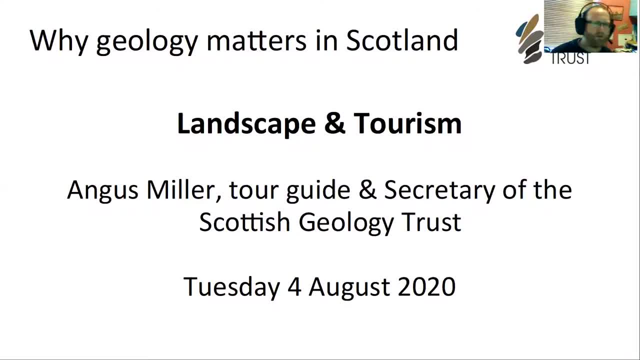 wide-ranging and dealing with overseas visitors as well, and what I'd like to just sort of explore today is what the issues are with getting across to visitors- whether they're visitors from the UK or from overseas- kind of getting a handle on Scotland's geological story- what's happening in the moment and what the potential is to do more. 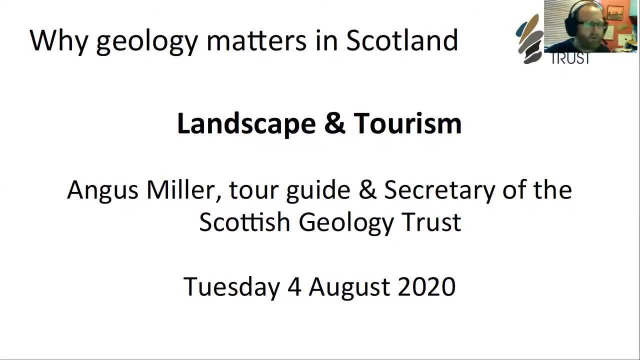 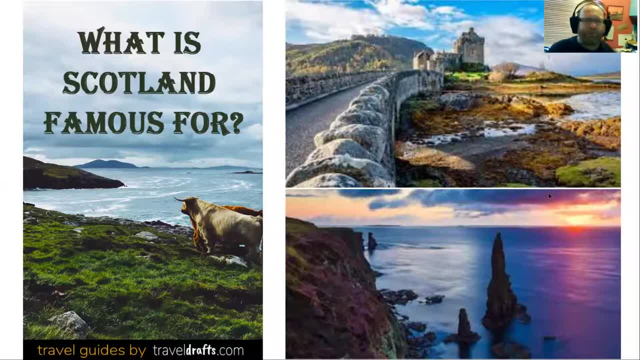 and really you know well what's the problems. is everything rosy and well? a kind of starting point, I suppose, is: why do people come to Scotland? what are visitors coming for? and if you do a quick google search for well, what is Scotland, you get lots of beautiful pictures of scenery. 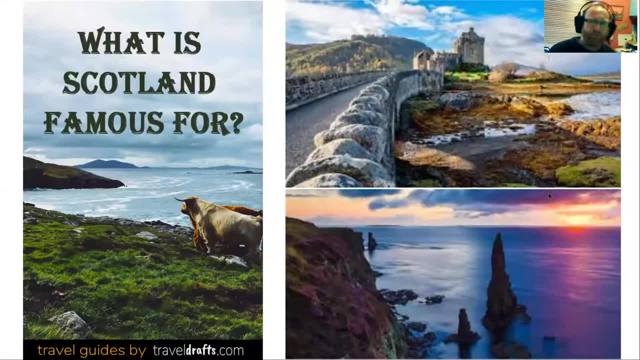 and we know from visitor surveys going back decades that scenery is the draw for Scottish tourism. it's the number one. Highland cows have quite a starring role as well, but it's mainly, it's mainly scenery. but of course it's not just the look of the land what really appeals to. 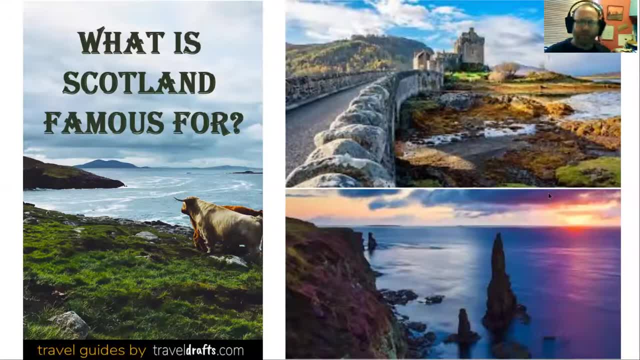 people is the castles and the human connection with the landscape, and a realisation that this is a landscape which has evolved through geological processes but also had a profound influence and input from the people that have lived in it historically and the people that live there today. so Scotland has a great package which, until this year, was doing fantastically well. 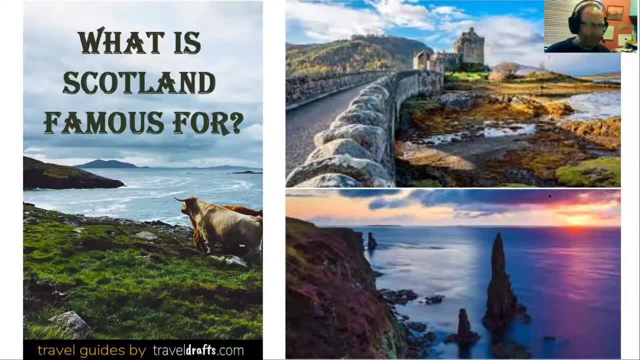 in growing tourism and the tourism figures have been going up recently and, associated with that, starting to get issues in places like Edinburgh and Skye with too many visitors at peak times and issues around that. but we've got a great product there and it's based on our scenery but it's much. 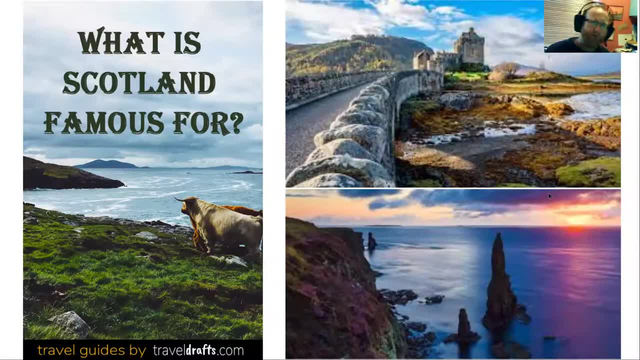 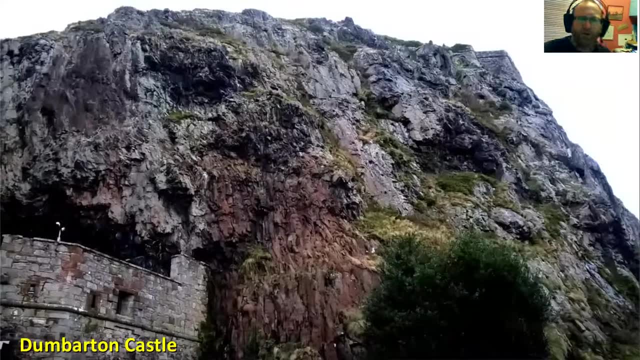 more multi-dimensional than just being about scenery, but I don't think it's really particularly about geology. so if you go to a place like Dumbarton Rock- the castle sitting on top of the rock there, really popular visitor attraction, and there's many, many like this around the country. 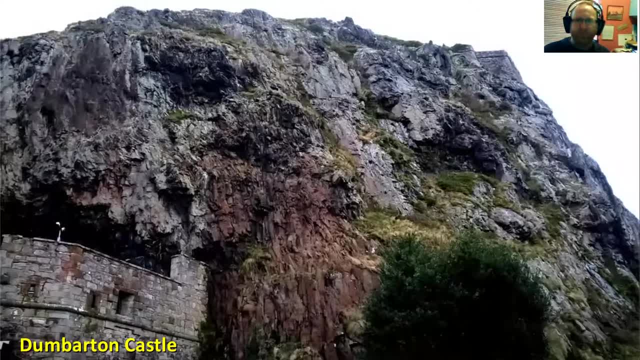 and, of course, a geologist looks at this and sees the volcanic plug and connects it with volcanic activity in the past and the story not just of the volcanic activity but also of erosion of this landscape, so that the contrast between the harder volcanic rock has come out from the surrounding softer rock and you've got a chunk of rock which is shaped. 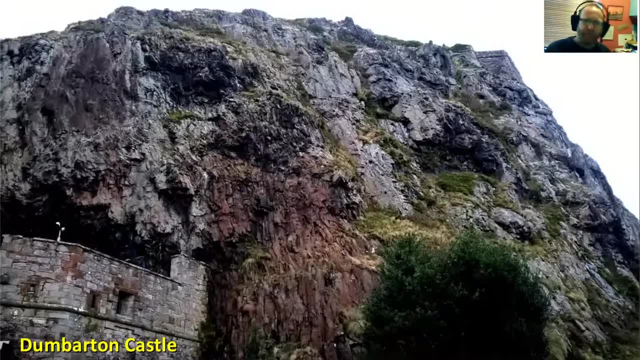 in a particular way by these geological processes and then has been used, been useful to people. so it's a rich story and if you go there you will find information. it's very superficial level about the volcano. it does mention it was volcano when it erupted, but what sort of used me about? 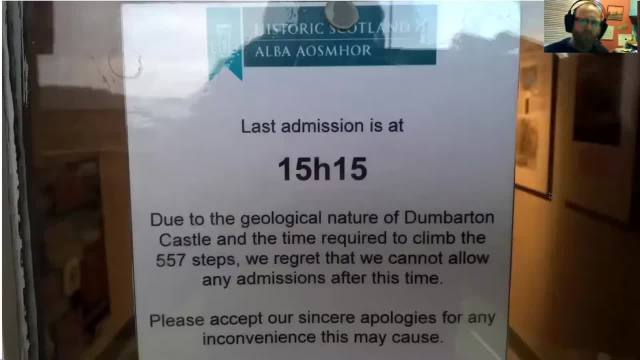 Dumbarton Rock is this notice last winter blaming the geological nature of the rock for the reason for closing early to allow people to clamber back down the horrible steps that they had to go up. and I'd like to present today a vision where the geology is maybe not seen as so much of a problem. 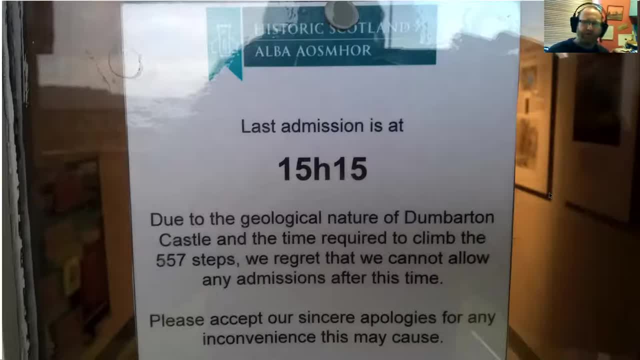 but is actually a part of a sort of a solution, and so it's seen as a very positive thing that actually we should be paying more attention to this geology and giving people information about it for everyone's benefit, not just for the tourist benefit, but actually for the local communities that are relying on. 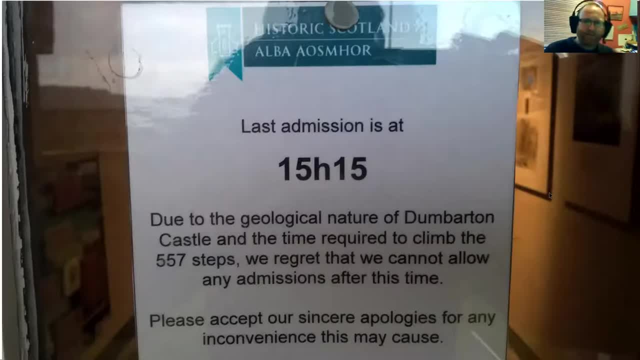 that tourist income and looking into coming decades. you know Scotland's doing great at the moment, but where's tourism going? what's it going to be like in 10 years and 20 years? I think there's a big case to be made to for doing doing better at talking about our 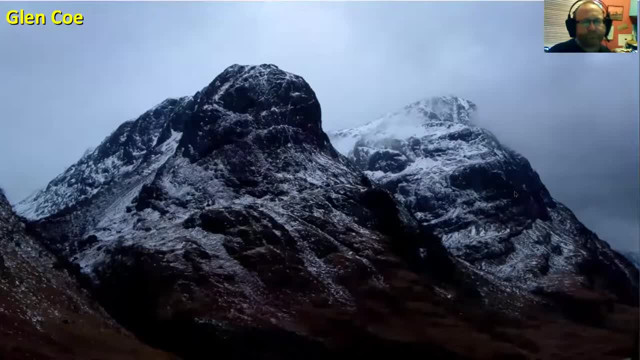 geological heritage as part of what we talk about. and another really good example is one of the big tourist attractions in the highlands, Glencoe did. I see we've got experts about Glencoe's geology here, which is very nice, and I, of course visitors in Glencoe are overawed by the scenery and the human story of the massacre. 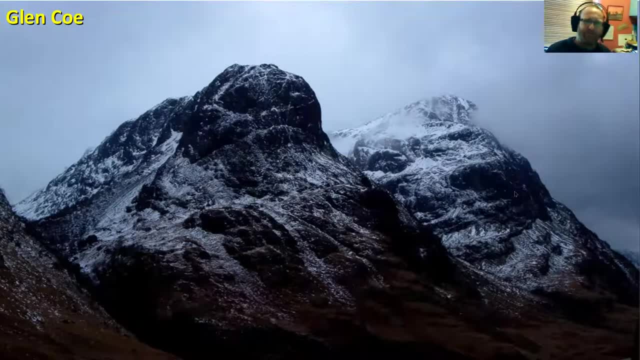 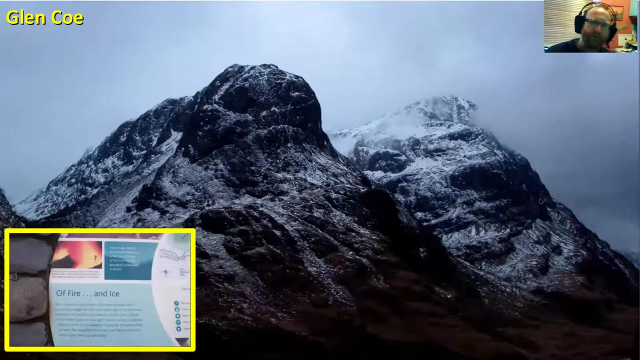 but I think there's a missed opportunity because geologically it's a fascinating story as well and if you stop by one of the big car parks in Glencoe you'll see information boards that tell you about the scenery and tell you about the volcanic activity, but they really kind of miss the mark. 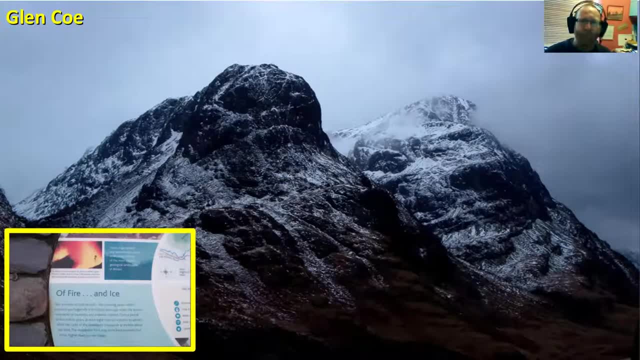 in terms of actually getting the wow of that story across in the scale of the volcanic activity that's there, and they also miss the chance to kind of say, but this is different, that actually Glencoe as a glen looks the way it is because the volcanic activity that's been preserved there is different from a lot of. 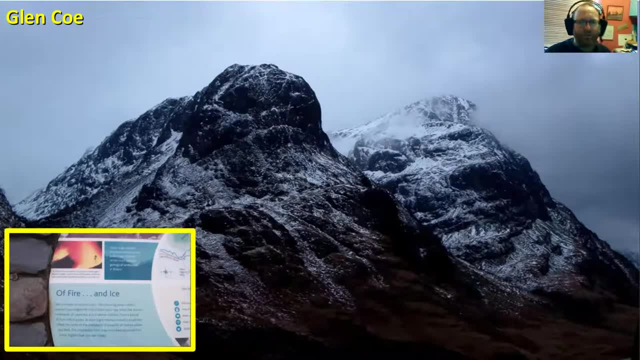 the rest of the highlands. and so when we talk about geological information, I think geologists of course are really keen to kind of get the detail in there, but I don't think we should lose sight of the big picture connections, uh, with what uh visitors we've got that are there. 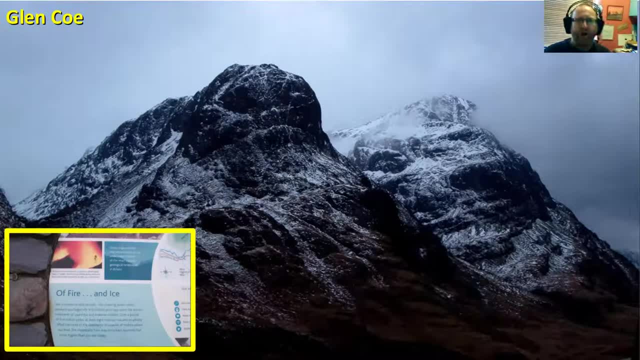 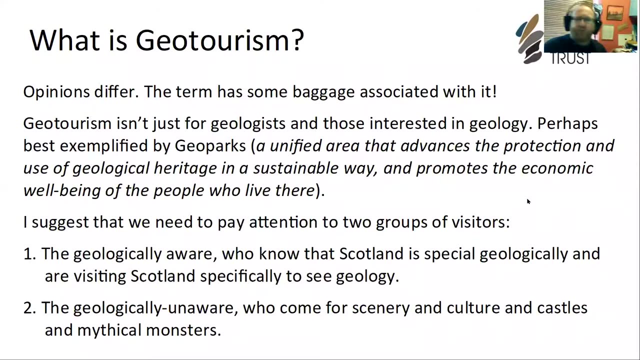 what visitors will actually connect with and be able to understand, and what they see and what they experience. So the term is geotourism and unfortunately, as with a lot of these things, you get different kind of interpretations of this and I'm certainly not going to want to get 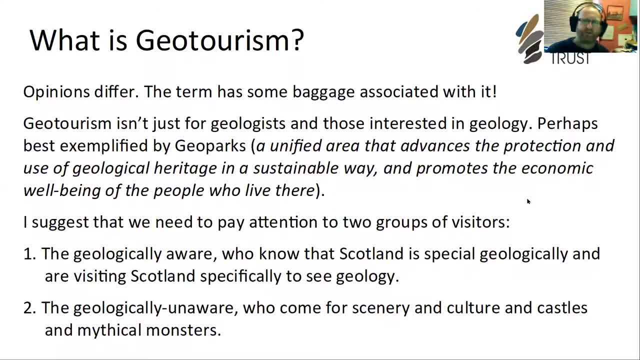 dragged into a conversation about what geotourism actually is. Frustratingly, the National Geographic took an existing term that was being used in a very particular geological context and applied it to a much more ecotourism, local community connection type of theme that they 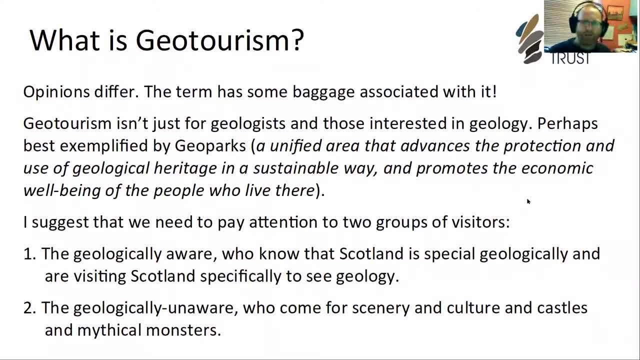 wanted to develop. So that's one part of it, but the other part of it is what geotourism actually is, who it's for, and so I think maybe in Scotland, the best thing for us to do is take a lead from the geoparks, and there's another kind of worms, if you like, in terms of 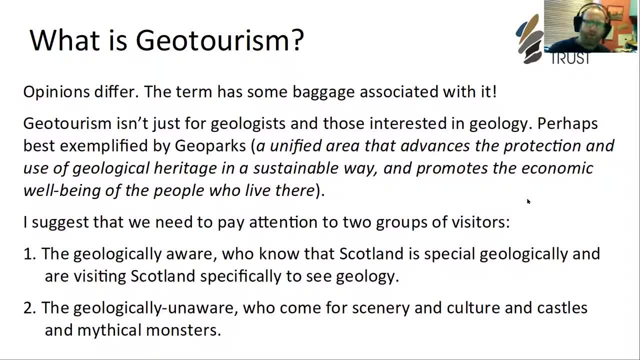 definitions. But geoparks are about local communities recognising and using and conserving their local geological heritage, So bringing in visitors, explaining about the landscape and the geology and making economic utility from it. And geoparks also have that very strong. 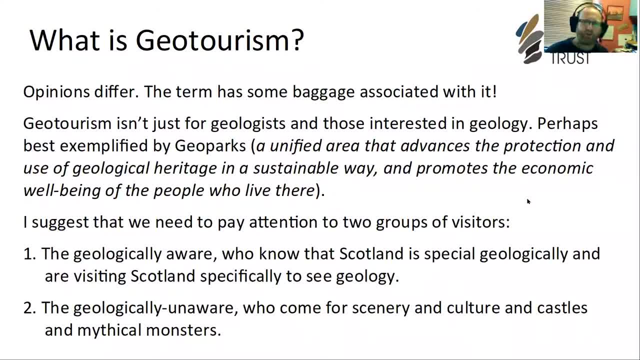 sustainability message about understanding how the earth works. So I think in its broadest terms we can look to a future of Scotland where people have got a better awareness of the geology of Scotland. But it's not just necessarily for its own sake, just about understanding. 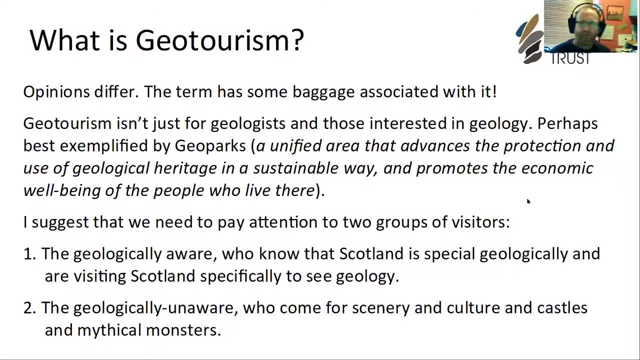 rocks. but it's about that kind of wider appreciation of how that geology fits into Scotland And how the sustainability issues and climate change can be learned about and understood through our appreciation of the geology as well. So in terms of the work I do and I think that kind of broader 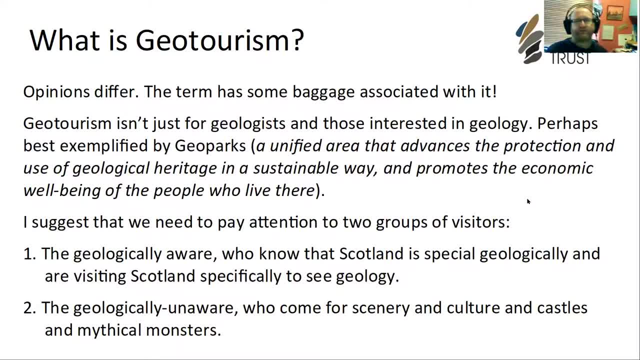 sector. I think there's a couple of different, there's two different strands really to geotourism And I think that both of them have got really interesting potential. Firstly, the geologically aware: the people that already coming to Scotland know a bit about geology And we're not just 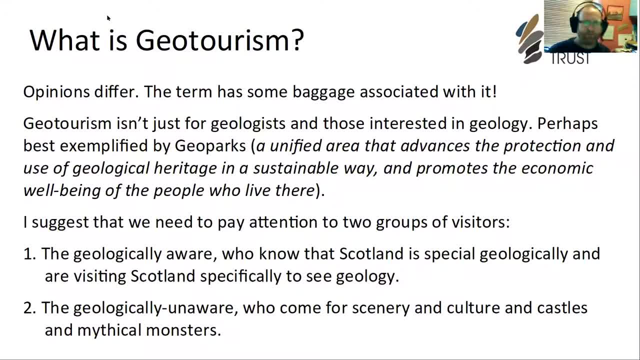 talking about geologists. There are hundreds of thousands of people around the world who don't have a geology degree but are really interested in geotourism. So I think it's really important that people are interested in the subject And they often know about Scotland already. They recognise 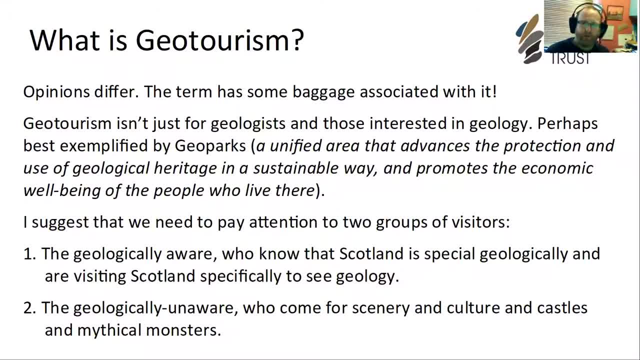 Scotland as being a place which has got really special geology. And they come, they already are coming, And well, who knows, who knows what sort of numbers, and that's one of our issues perhaps. But golf tourism, for example, is really recognised in Scotland And there's statistics about how many. 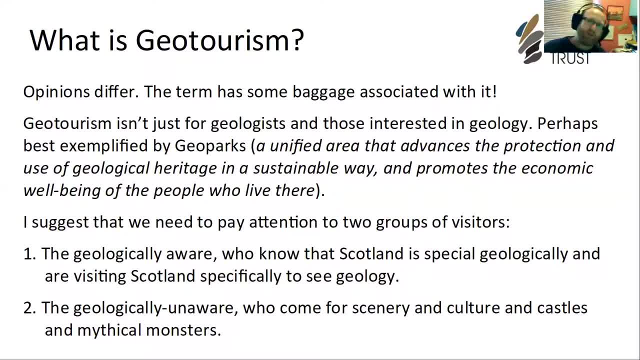 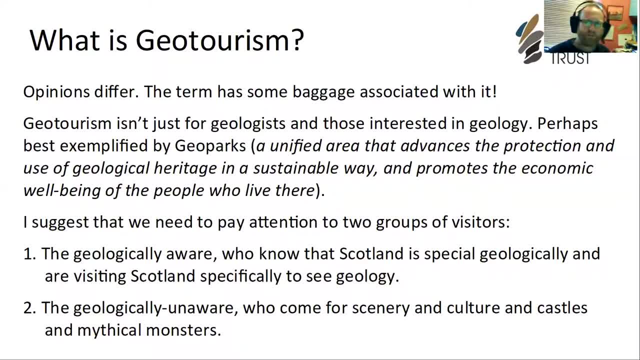 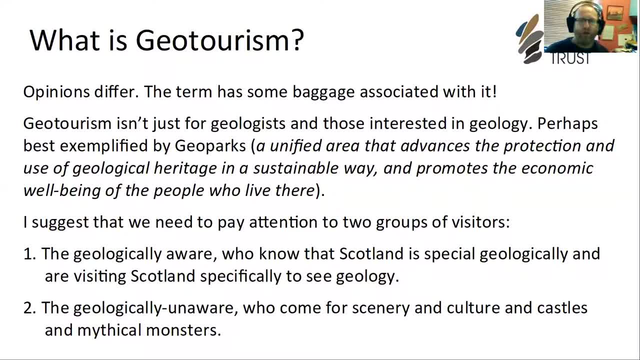 who claim not to be at all interested in rocks and roll their eyes whenever I mention anything about geology. But I think for that kind of less interested visitor there's the opportunities to make the connections with the big stories as I was talking about earlier in Glencoe and kind of. 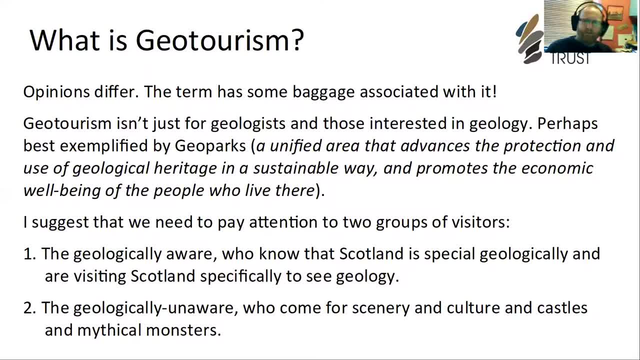 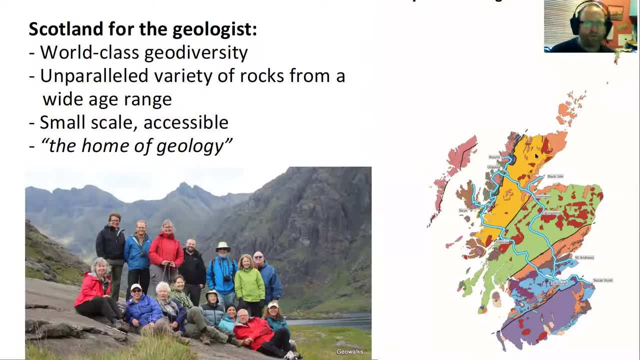 bring make the connection between the bedrock and the processes of the past, with how the landscape looks today, the human story of that landscape and looking forward into the future. So first of all, Scotland for the geologists, And I think there's huge potential here. I've 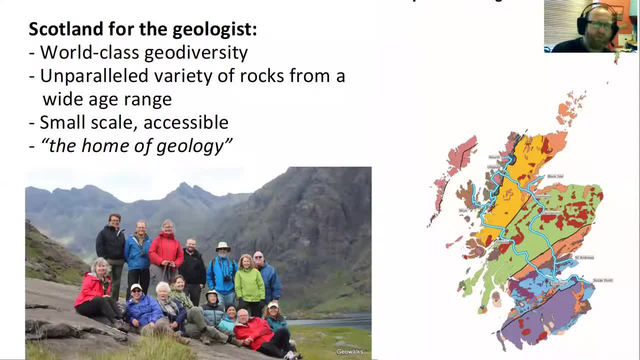 done a little bit of engaging with international visitors in this case, and one very successful enterprise that I've been running for about almost 10 years now is with a Californian organised organisation, actually a Californian geologist who comes now every year to do a 12 day or a 14 day. 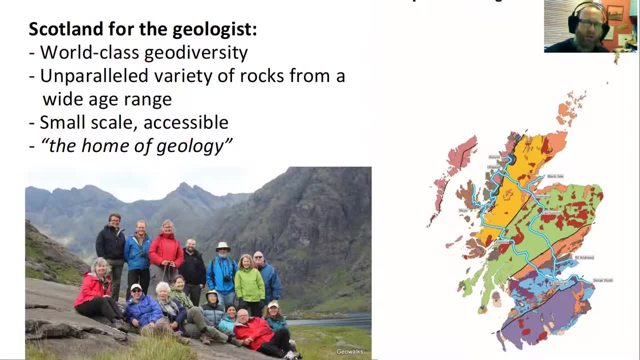 tour of Scotland And we've now developed three different sort of two week itineraries. This is the map shows the first one, which is the kind of geological highlights, and they go to Sickerpoint and Edinburgh and St Andrews and up to Inverness and the Black Isle over to Allapur and Ascent. 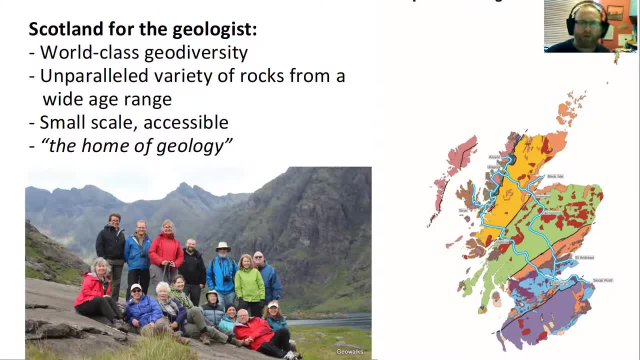 and then down through Skye and Lochaber and Van Buren And back to Edinburgh And it's a fantastic kind of 12 day tour And we get geologists mostly from North America coming on that and really soaking up this amazing geological story. And what I've got. 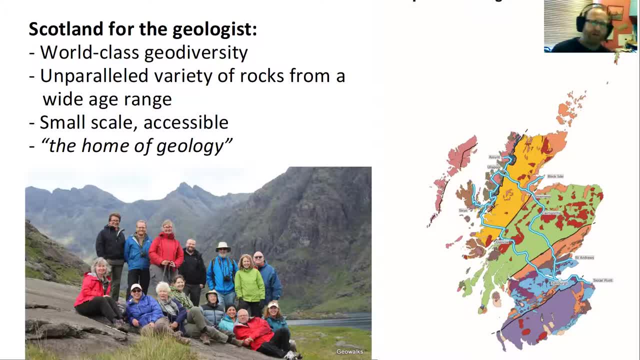 from these sort of tours is that, yeah, Scotland's geology is great. There's the landscape and the rocks. I've got an interesting story to tell And you don't get you know. you don't get you know. 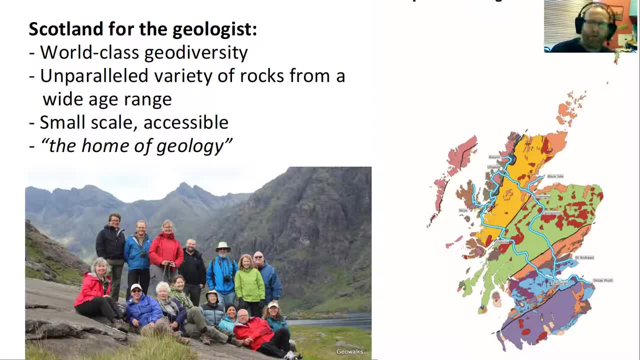 this sort of scale of geology very commonly elsewhere in the world where there's so much variety in terms of different rock types and the age ranges, And it's very easy to travel around. So and that sort of trip. we try and minimise the amount of time we're spending in the coach. 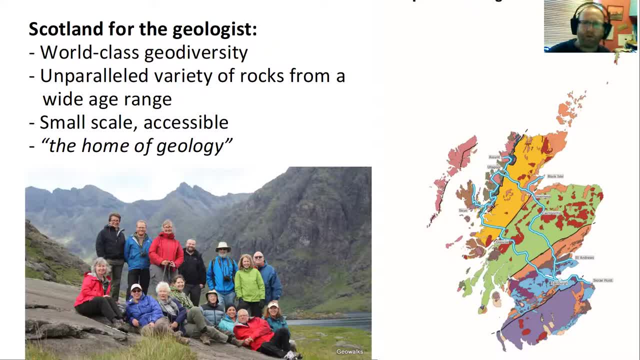 and getting out every day and walking for a couple of hours, And so over that 10,, 12,, 14 days, you get a really nice range of scenery, rock types And different geological stories, plus seeing the very strong connections into everything else. 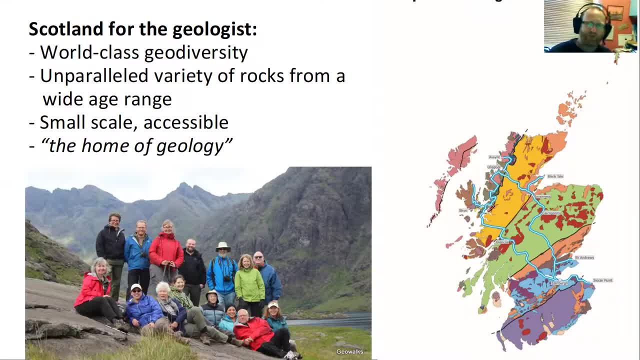 So we've got something to sell. We've started using this slogan: the home of geology. I invented it and discovered that nobody else was using it, So we started using it on the Scottishgeologycom website and it's now there. we've now got it, So officially, Scotland is the home of geology. 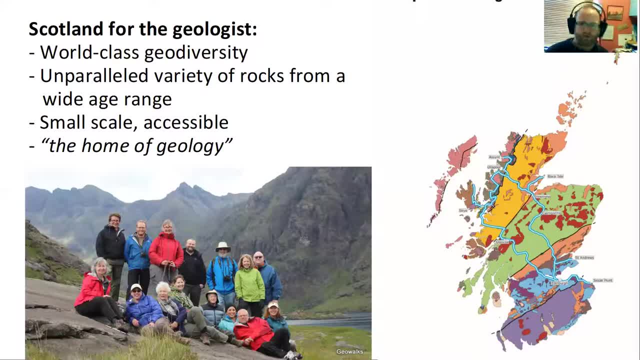 And I think that's something we can market around the world. We should be making more of it and bringing people from abroad specifically to say, yes, this is it. and of course, I haven't mentioned yet about the birthplace of geology and James Hutton and so many other lines of geology which. 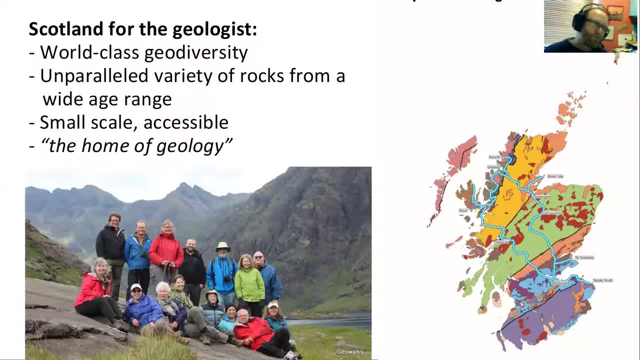 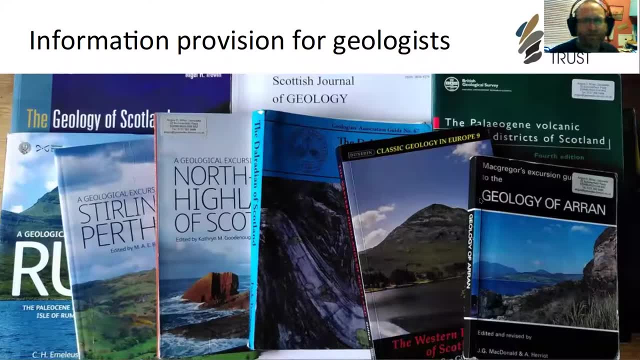 have developed from places like Glencoe is another great example. So there's lots there which we can make use of. So what do these people need? Well, if they're a professional geological party doing a field trip, there's a huge amount of information available, a lot of really good information. 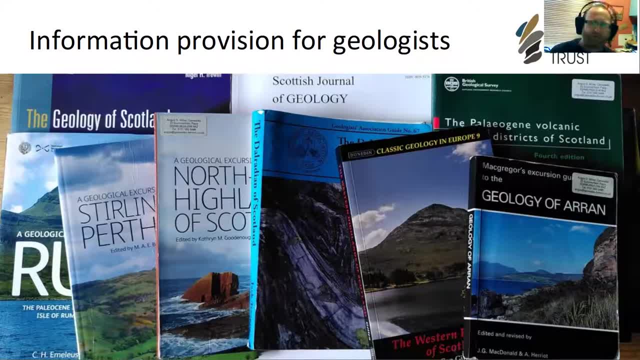 very wide ranging, and this is just quick selection from my bookcase, and there's a range there. there's some stuff that's 20-30 years old, there's some stuff that's just been published in the last year, but this stuff's really accessible and, of course, as well as the physical printed books and excursion. 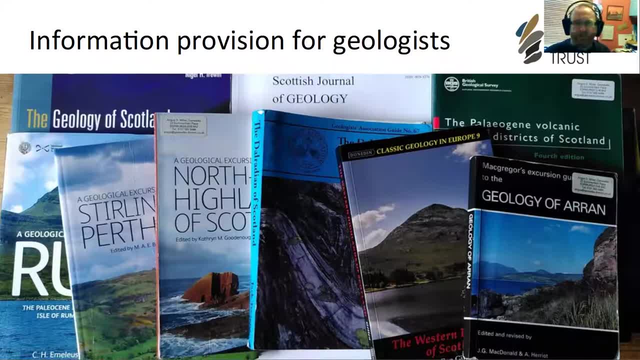 guides, there's a lot of academic papers and certainly recently a lot of stuff that's been published with very clear images and photographs and grid references. so it's really easy to take a paper if you, if you know geology, and to go and see some some really good stuff. so in some ways, 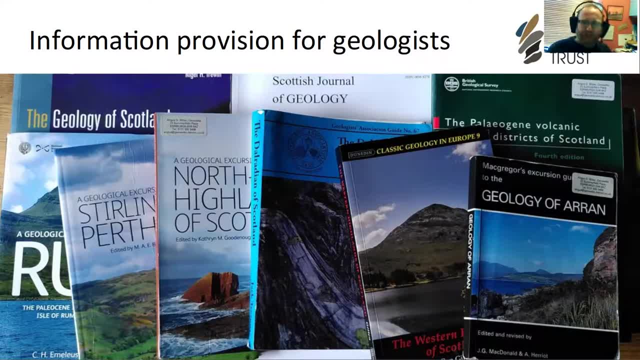 to sort of support this industry, if you like. um, there's a lot of information there, but how do you find that? uh, how to make it easy to for overseas geologists to say: oh look, you know, this is where i can put together a really nice uh field excursion and go and visit, or i'm a tourist. 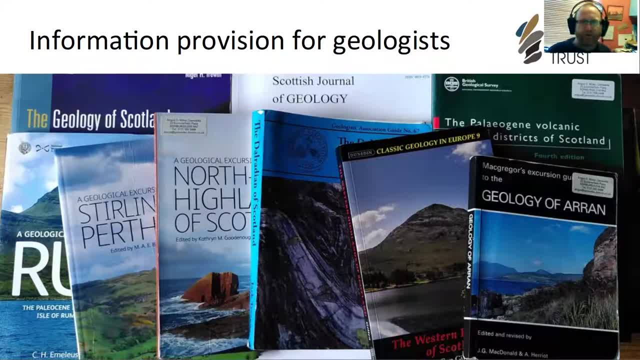 a geological tourist from another country. i've studied the geology in my country. i wonder: uh, you know, kind of go to scotland and easily find my way around and and i'd see some great geology. i think the answer is yes, but it probably needs uh. uh, there's always work to be done and 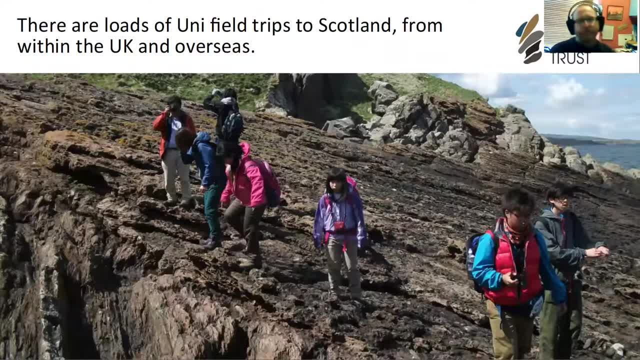 making that more, more easy for people to do. there's also the university sector, and i'm not going to say too much about this today because i'm trying to line up a session for maybe two or three weeks time, uh, where it'd be great to get some, uh, university researchers. 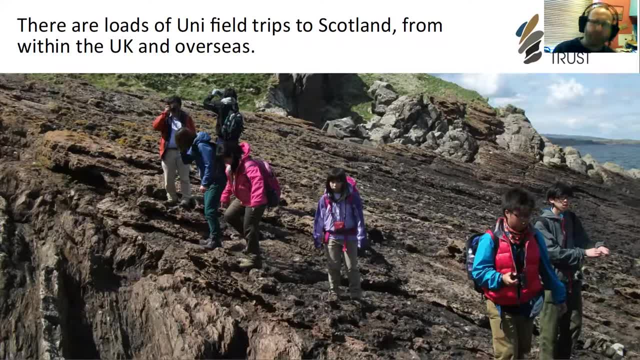 uh, particularly people that are organizing field trips, and to talk more about this issue and the the connection of the kind of university sector with uh with scotland's geology. but a little bit of experience with that and this is a group from tokyo city university and japan. 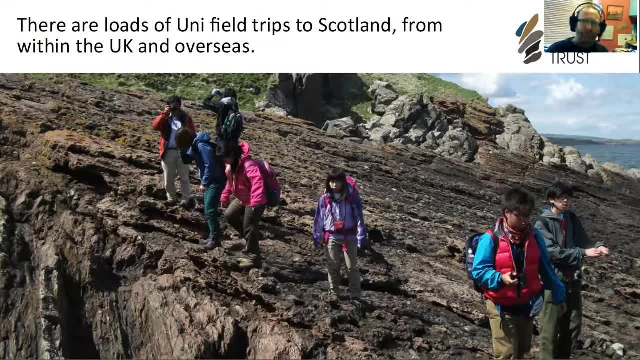 and they come to scotland every year and of course they're coming for that range of rock types and ages and processes that you don't get in japan. you uh, and they are self-led, um, and they get around by public transport and they really show what. 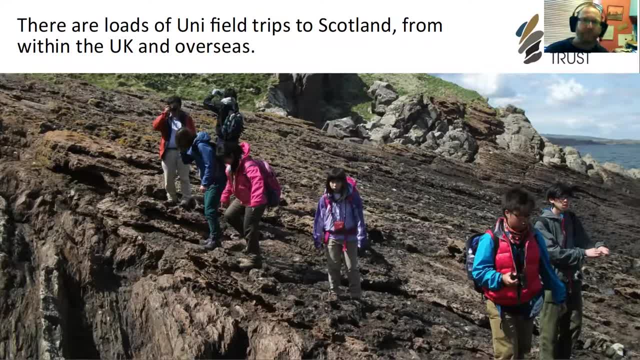 can be done and to get to some really wide-ranging places. uh, and they are always so enthusiastic about this and they've got good connections with uh people like john faithful and uh and glasgow university in terms of uh ongoing research as well, so it's a really nice connection, but it's 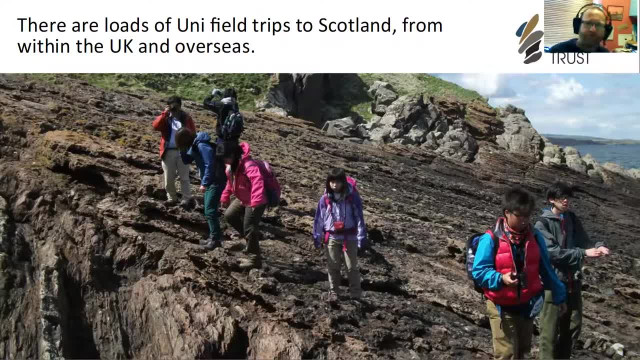 fundamentally about bringing students and showing them a range of good geology and they see scotland as being absolutely uh ideal for for the future and i think that's a really good connection for that uh circumstance. and, of course, that picture i'm sure some of you will recognize as as a 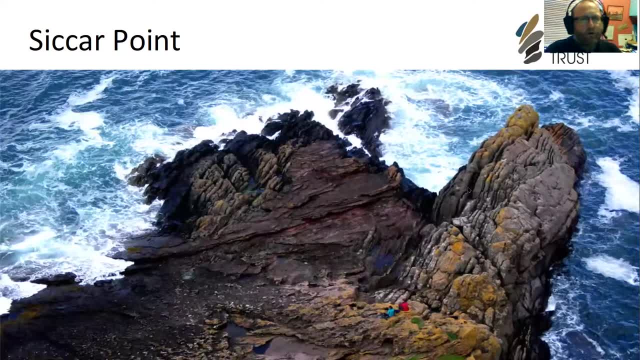 sicker point because i think for geologists of course, seeker point is really well known. it's probably the most important geological site in the world- you can argue about that, uh- but there's no doubt that it's very often included in university curricula. it's often talked about in high schools. 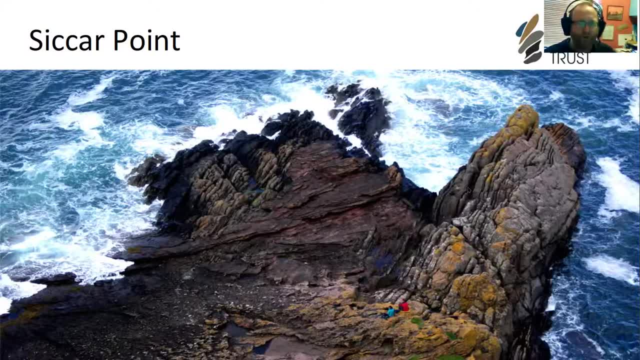 discovered, not in Scotland, of course, that would be too obvious- but elsewhere in the world. people learn about James Hutton and they learn about Sicker Point. So it's a very interesting and beautiful site and there are issues because it's at the bottom of a steep grassy slope and there's a lot of universities, aren't? 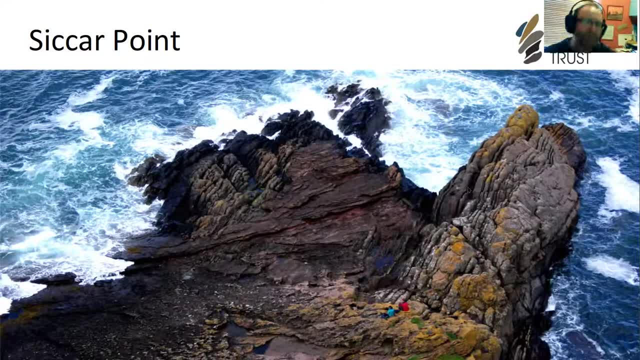 too keen about taking students there because of that, so there's definitely issues there. But for anyone who's interested in geology, we've got this beautiful site with clear unconformity, a very clear connection with the development of geology as a science, and the nice thing is that you 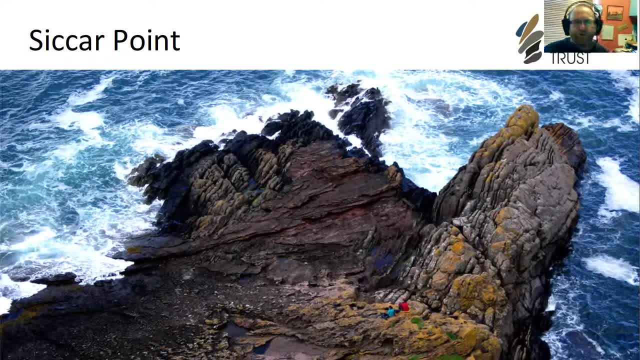 can go there and you can see today really as it was when James Hutton discovered in 1788.. So it's a very kind of evocative place to imagine the development of ideas. but it's also more than that, because it's that connection. 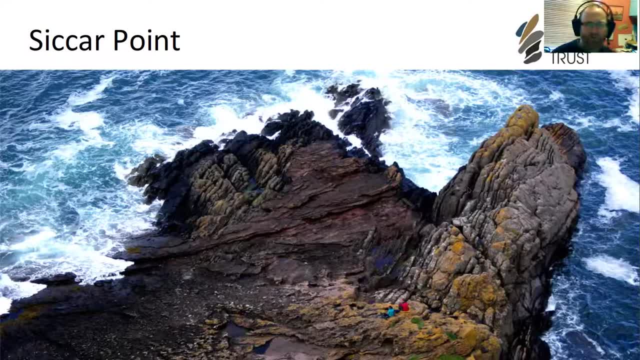 between the Southern uplands and the central lowlands of Scotland and you can see the geology played out in the landscape roundabout. So it's got a great connection to the geology as well. great deal to offer, and I've shown you two pictures of it, One of it being busy. 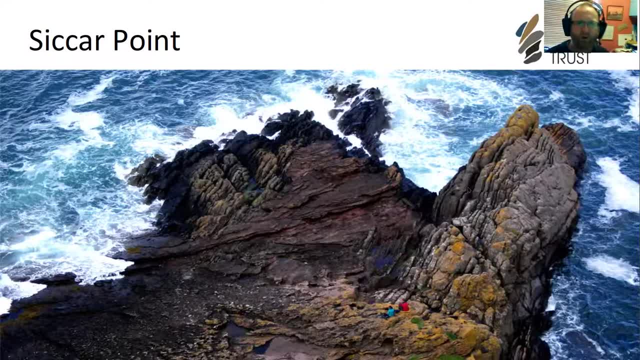 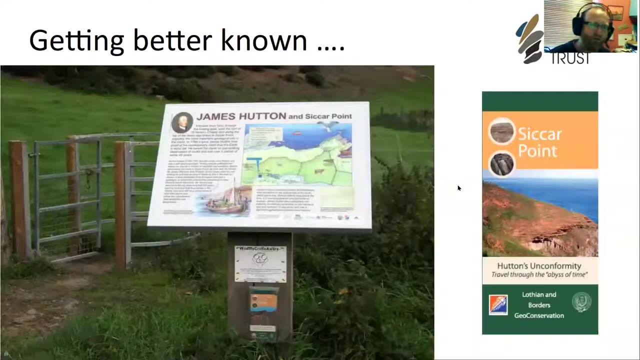 with a university group there, but it's much more common to go there and see nobody, or maybe just a couple of people there. Isn't that amazing about? you know one of the most important, if not the most important, geological site in the world, and you often have it to yourself. It's changing. it's certainly getting. 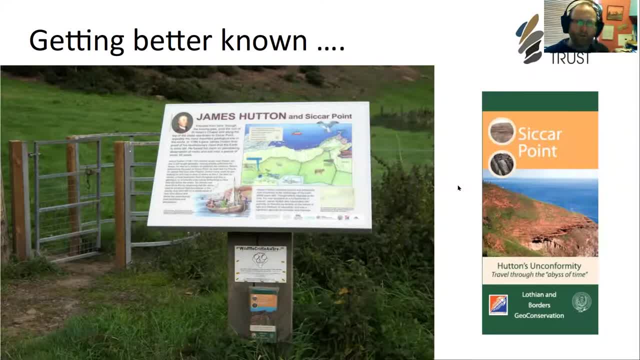 better known and it's nice to see that in the local communities there's quite a lot of awareness of that and there's been various projects over the last 10 years or so which have improved the information. So there's now a couple of information boards there. they've just been replaced in the last year or so and 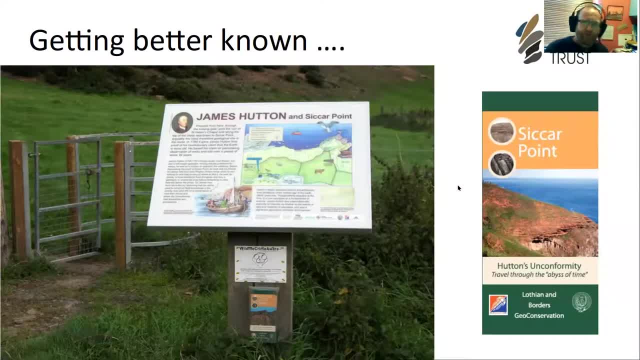 there's a leaflets available online and some good information online, So we're doing a bit better about shouting about sicker point, but there's still an awful lot of people in Scotland don't know that it's here and don't know about James Hutton. 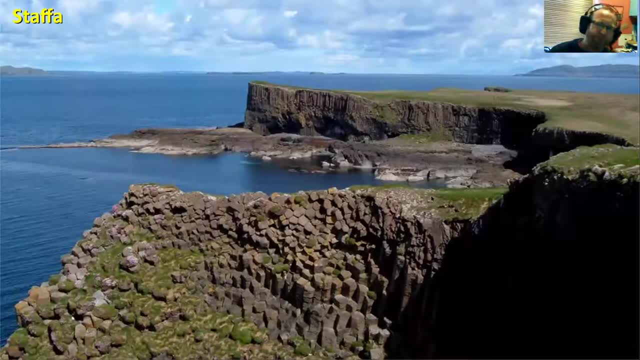 Thank you, And I think there's a really interesting contrast between sicker point and places like the island of Staffa, which is geologically stunning, of course, and has got an interesting history because it's been on the tourist trail for a long time and it's got this connection with art and music and, if you 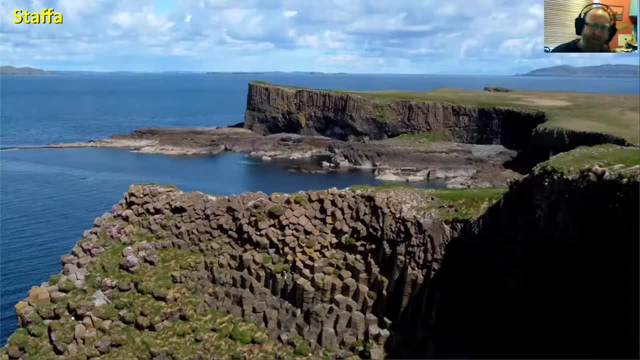 go to Staffa today. well, it's usually got a couple of hundred people scrambling around on it and the boats are zipping backwards and forwards and it's really interesting Why has Staffa got boat trips and a huge draw, whereas places like sicker point haven't? I don't. 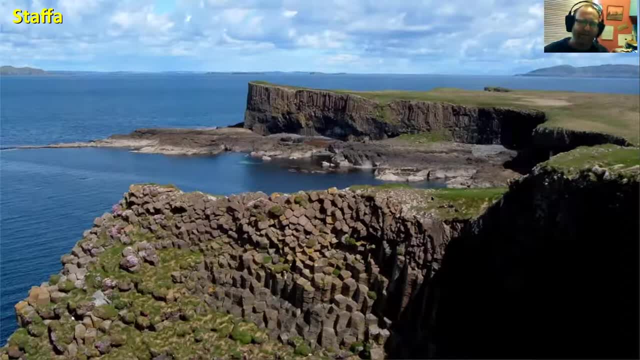 know why, but I think there's certainly an issue there that we could help address, because both in terms of bringing people to other places and other parts of Scotland, where there's interesting geology to be discovered and interesting connections of people, but also in places like Staffa, so that you know, there's a lot of people who are interested in that. 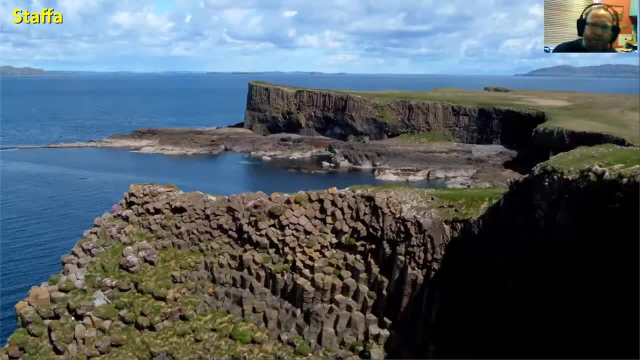 The visitors that go there do get some sense of geology, and it is there. There's lots of information if you search for Staffa geology, but it's often quite technical and it misses the kind of wow of that big story of the development of the North Atlantic and volcanic activity on a huge scale on. 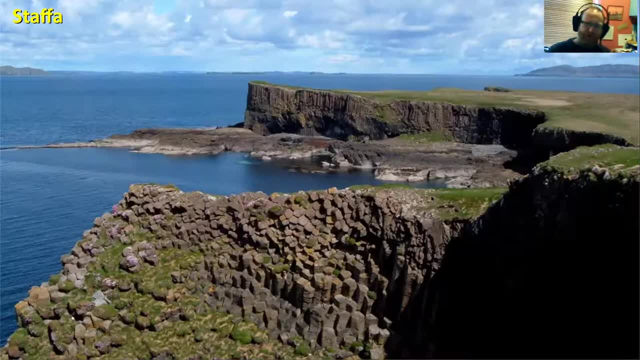 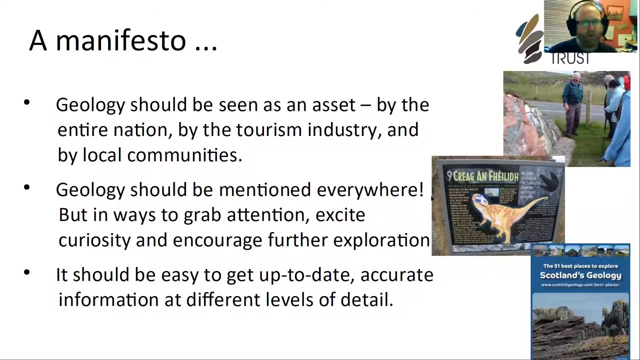 the West Coast. Sometimes it's too much focusing in on the detail and missing the big picture, So I'm going to stop, but just a couple of last slides. I think my kind of personal manifesto here is to say that I think that Scottish geology. 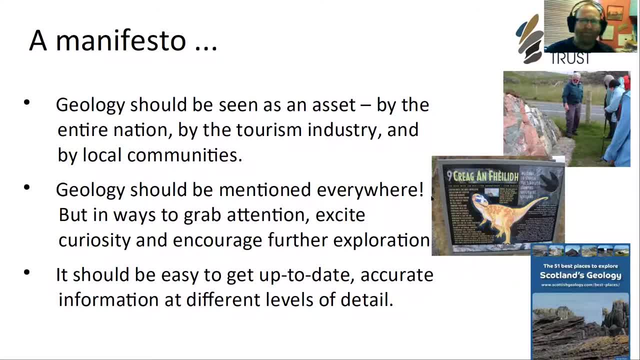 should be seen as an asset. I was joking about Dumbarton Castle and it being seen as a hindrance and liability. but why aren't we making much more of that so that Scotland as a nation recognises that our geology is important and special, that the tourist industry makes use of this and we bring people, arrange a? 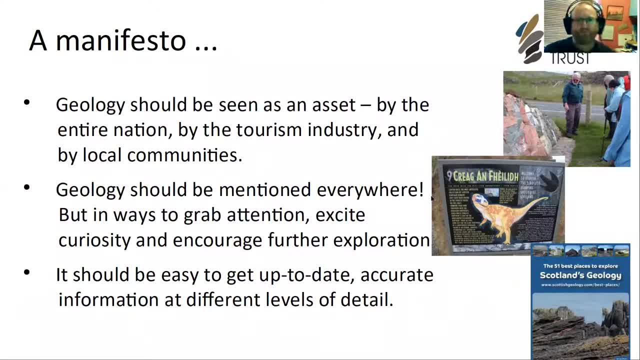 people coming for the geology specifically, but also people that are coming for the landscape, get a richer experience because they get to see a little bit about, learn a little bit about why it looks the way it does, and for communities across Scotland to spread the tourism industry out a bit. 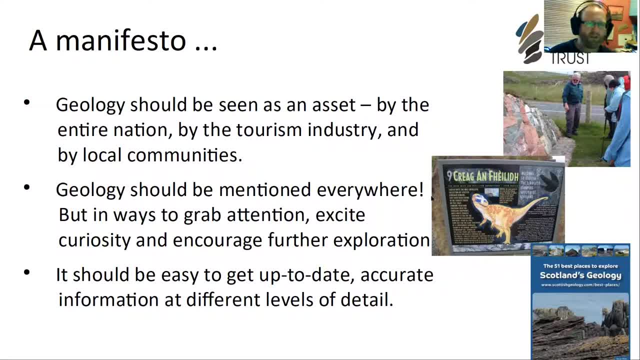 and to actually get people going to other places. and so what I'd like to see is that whenever you stop at a little visitor center or an interpretation beside the board, beside the road, or you you're in a coach and you've got a excellent blue badge guide at the front with the microphone, that in all of these 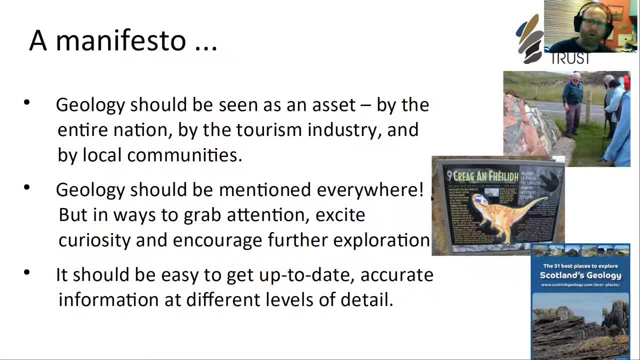 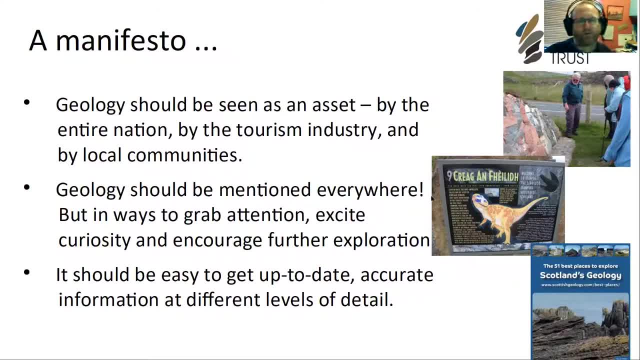 there's some good, really great stuff going on about the dinosaurs, for example. people love dinosaurs and that's a great way of getting people interested and so we tell people that some of the story we excite them, we get them more interested and then, when they are more interested, it's really easy to find that deeper. 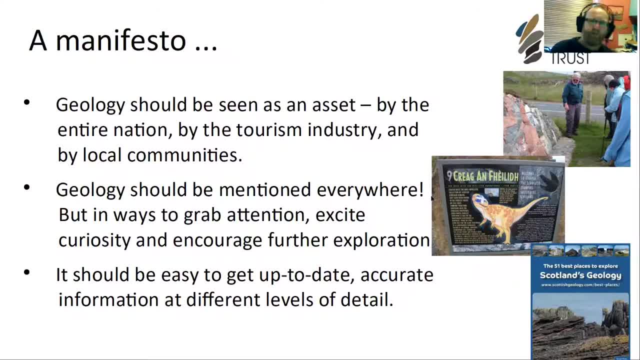 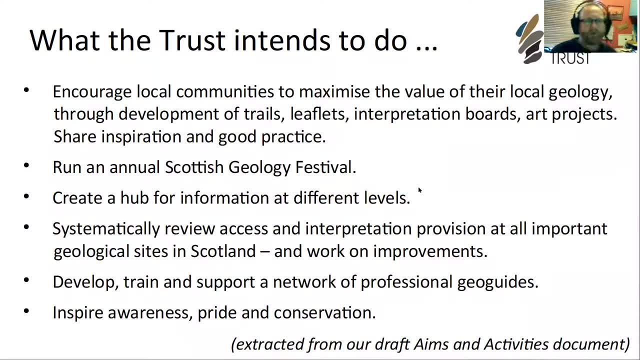 level of information, that is, it's easily available, that it's up-to-date and that people can go as deep as they want into the subject. well, the Scottish geology trust is. we've got a draft document, aims and activities. it's been circulated to people that have been involved in the 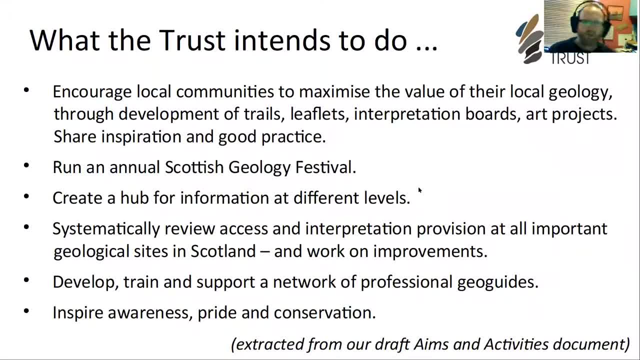 trust activity so far. if you'd like a copy I can send you out. but just in terms of the tourism aspects of things, this is kind of some of the things that we would like to do is encouraging local communities to maximize the value of that local geology, to use it to bring visitors and to benefit from that and that there's. 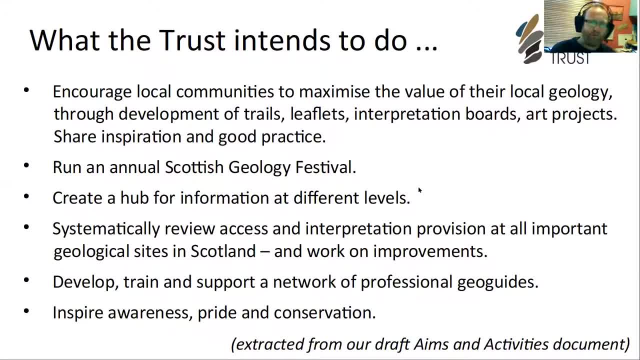 lots of different ways that that can be done, whether it's physical things or the ground which are telling people about it, but also that kind of wider way of what actually the geology is intrinsic into the landscape and culture of Scotland, and so what we'd like to do is to is to facilitate that and to share good. 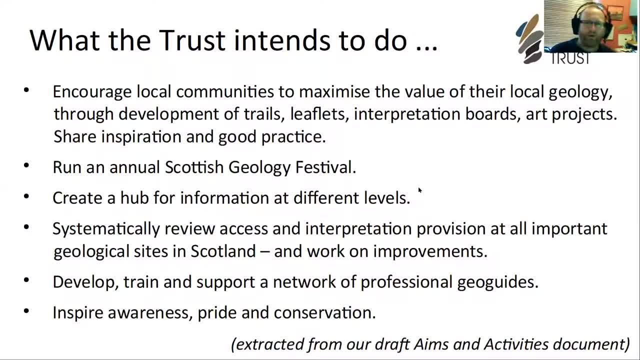 examples and to encourage more. we are going to run an annual Scottish geology festival which will showcase these examples and encourage organizations and individuals to get involved and to get involved and to get involved in the world and doing more of that and and to create that information hub so that it 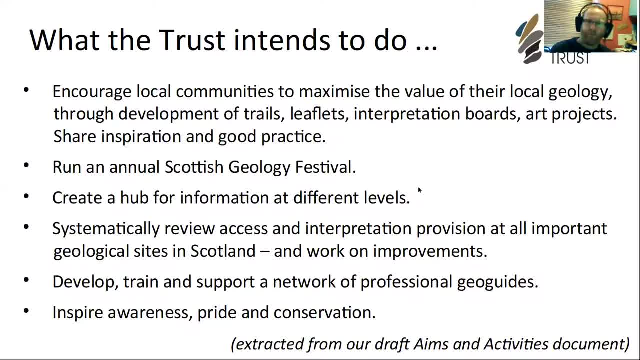 is easy to get excited about Scottish geology if you don't know about it and you're thinking about planning a trip. but also if you're here and you're wanting to get a bit more detail, you can even drill down into that and in the longer term, really, where our aspirations is, to balance things out of it, to say